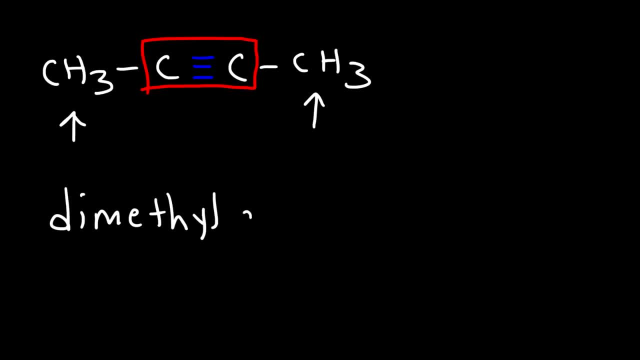 dimethyl acetylene, And so hopefully you're getting the hang of how to write the common names of alkynes. Now let's move on to our next example, which is going to be CH3CH2C, triple bond CH. So go ahead and write the common name for that alkyne and also write the IUPAC name. 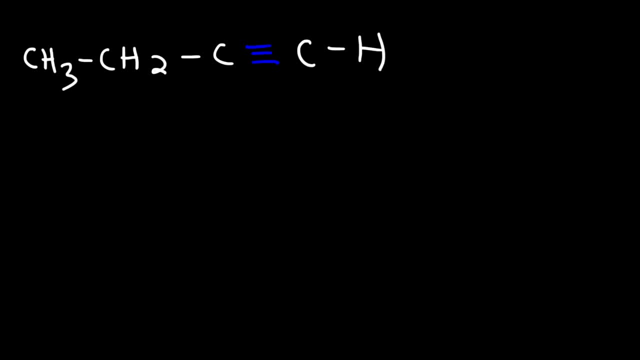 since we're here already, Let's go ahead and do that. Let's start with IUPAC name actually. So this is carbon 1, 2, 3, 4.. So 4 is associated with butane, but instead of writing butane, we're going to write butyne. Now the triple bond is on carbon 1.. So this is called. 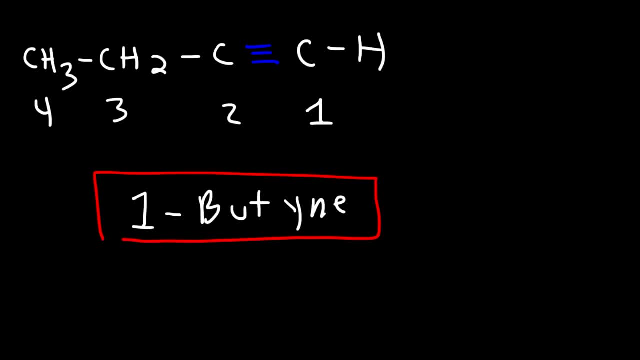 1-butyne. Now what is the common name of this particular alkyne? So we can see that we have our acetylene group and this is an ethyl group attached to it. So the common name is going to be ethyl acetylene, And so that's it for this example. 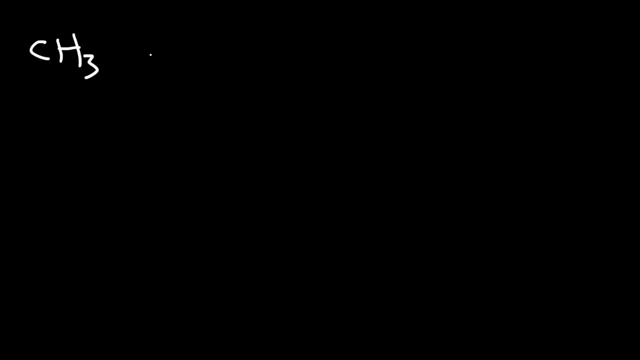 Here's another one. So for this example, write the IUPAC name and also the common name of this particular alkyne. So let's start with the IUPAC name. We need to number in such a way that the alkyne has: 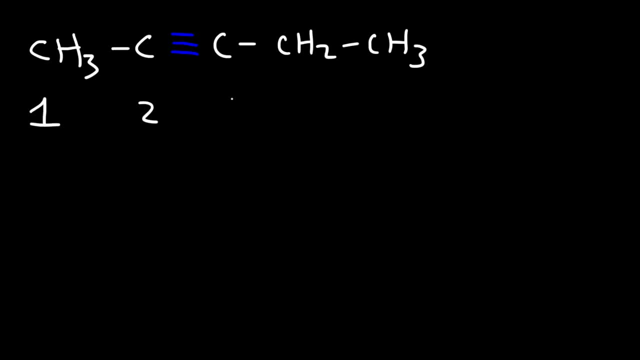 the lowest possible number. So this is going to be carbon 1,, 2,, 3,, 4, 5.. So that's pentane. But instead of saying pentane, it's going to be pentine. Now, the triple bond is between carbons 2. 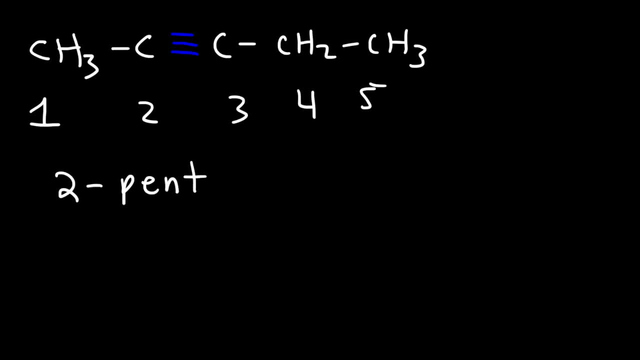 and 3.. So we have to pick the lower of those two numbers. So this is going to be called 2-pentine. Now let's try the common name. So here is our acetylene functional group, and on the left side we have a methyl attached to it and 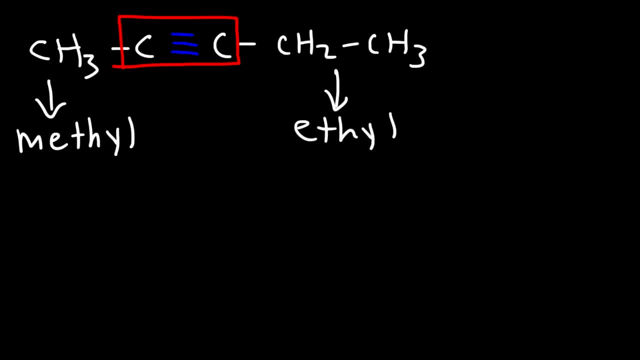 on the right side we have an ethyl group, On the left side we have a methyl attached to it and on the right side we have an ethyl group. So we need to put it in alphabetical order. So the common name is ethyl-methyl-acetylene. 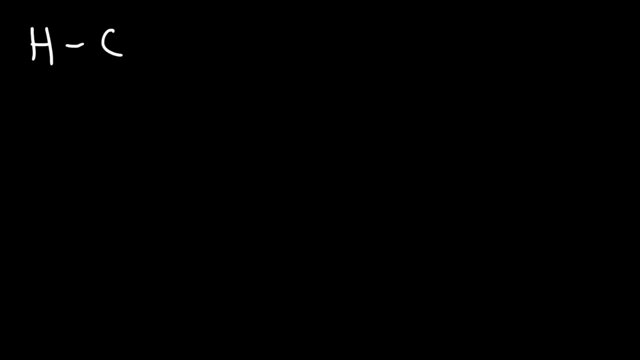 Now for this next example. all I want you to do is to write the common name. So let's say that we have a benzene ring attached to the carbon-carbon triple bond. How can we name it So? notice that whenever you have a benzene ring as a substituent, it's called phenyl. So to name this. 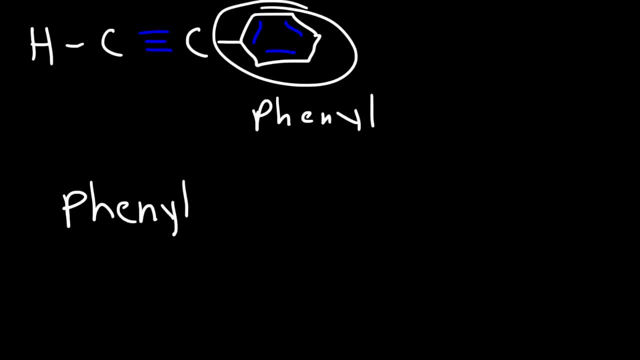 it's simply going to be phenyl acetylene, And for the common name you need to write it as one word. So if you see me put a space, it really should be together as one word. So just keep that in mind. Now let's work on another example. So for this one, write the common name and the IUPAC name. 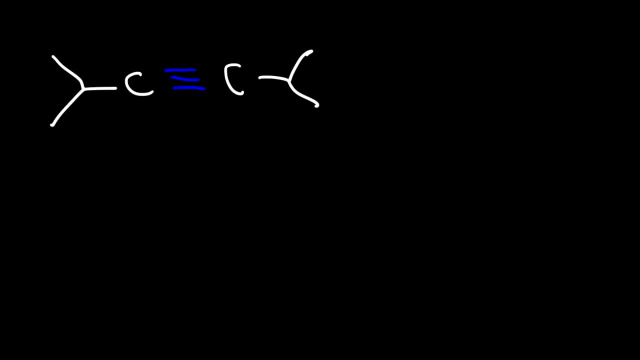 as well. So let's start with the IUPAC name. This is going to be carbon 1, 2, 3, 4, 5, 6.. So we have a methyl on carbons 2 and 5.. So it's going to be 2, 5,. 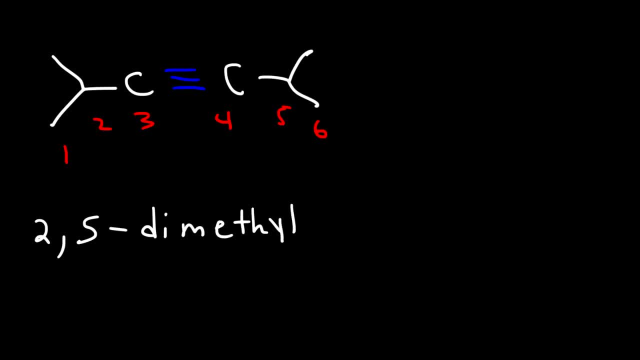 dimethyl, and for 6 carbons, that's hexane, but we're going to use hexime and the triple bonds on carbon 3.. So it's going to be dash 3, dash hexime, And so that's how you can name this particular alkyne. 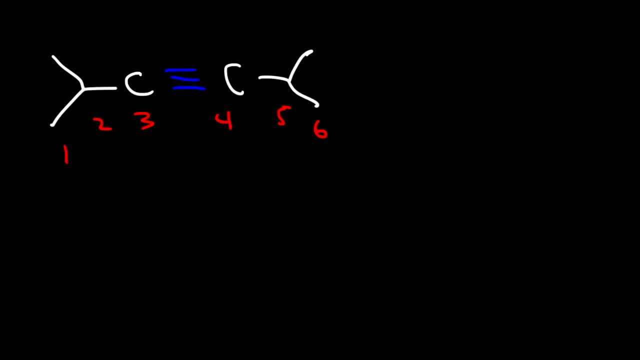 Now, what is the common name for this particular alkyne? It's the common name for this particular molecule. So notice that we have an isopropyl group on the left side and on the right side, So this is going to be called diisopropylacetylene. 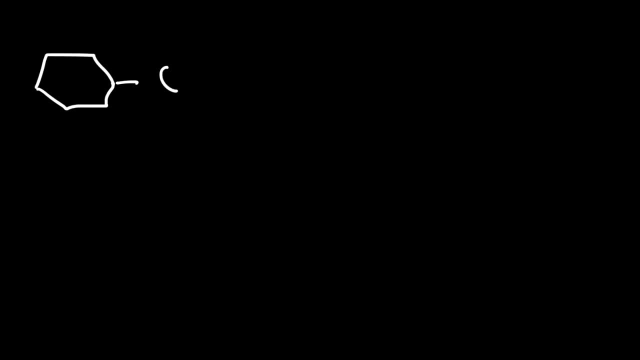 Now let's work on one final example. What's the common name for this molecule? So we have two phenyl groups attached to the acetylene part, So it's simply going to be diphenyl acetylene. Now let's work on some more examples with IUPAC nomenclature. 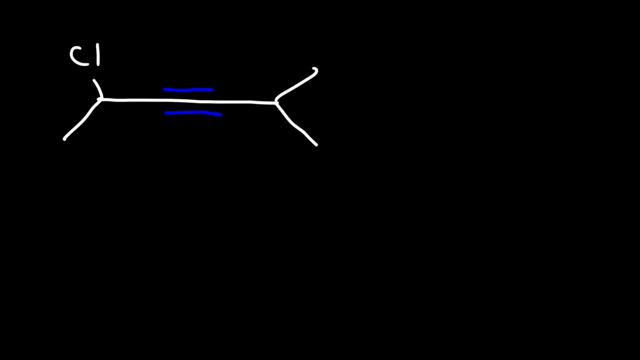 So go ahead and write the IUPAC name for this particular alkyne. Now should we number it from left to right or right to left? If we go from right to left, the triple bond will be on carbon 3.. And if we go from left to right, the triple bond will still be on carbon 3.. 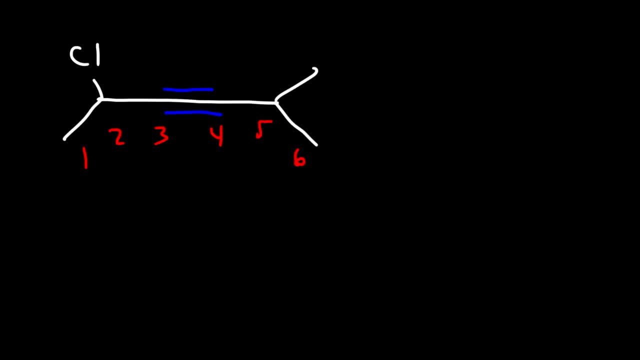 So which way should we go? Going from left to right, we're going to have the name 2-chloro And then we have a methyl group on carbon 5.. So it's going to be 5-methyl And we have the alkyne on carbon 3.. 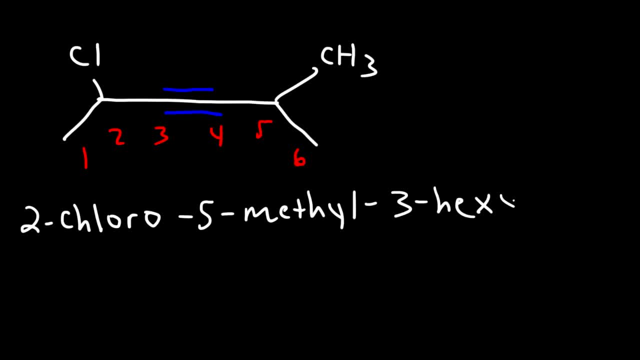 So that's going to be 3-hexime, because we have 6 carbons in the parent chain. Now, if we go in the other direction, this will be 1, 2, 3, 4, 5.. 5, 6.. 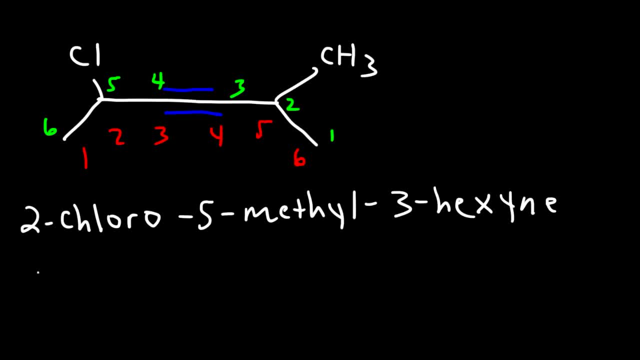 So chloro still comes before methyl. We still need to put it in alphabetical order, But it's going to be 5-chloro-2-methyl-3-hexime, And so the first one is going to win, because you want the first substituent to have the 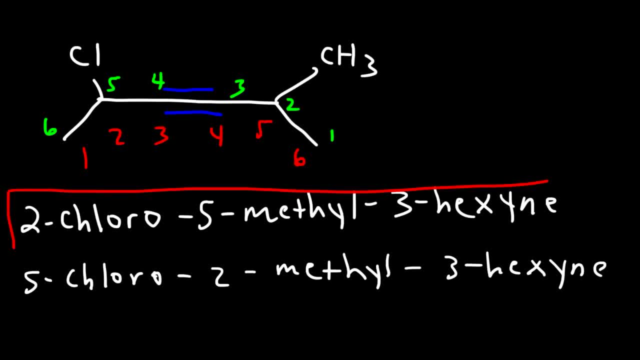 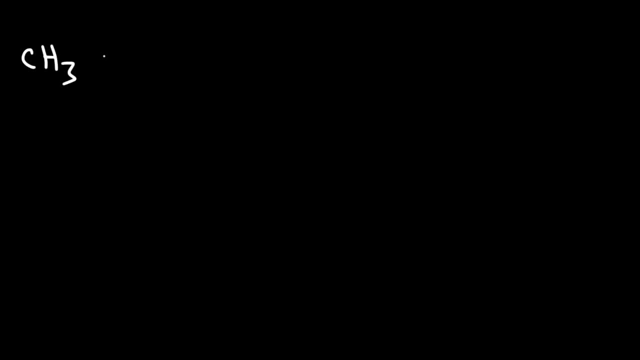 lower number, And so this is the right answer. Now let's move on to our next example. So it's going to be CH3CH2-CH with a CH3 attached to it, And then we have our carbon-carbon triple bond. 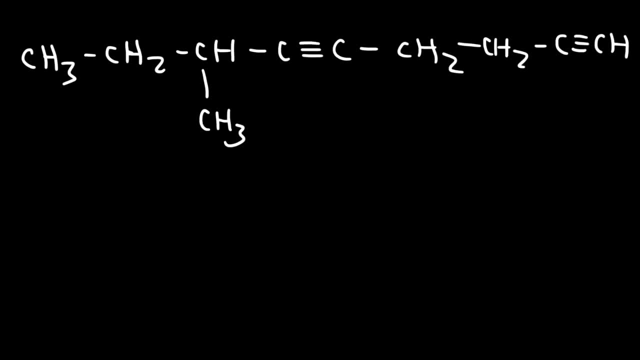 And another triple bond at the end. So go ahead and name that molecule. So, because we have the triple bond at the end here we want to start counting from right to left. We want to give the triple bond the lower values, So we have a 9-carbon chain. 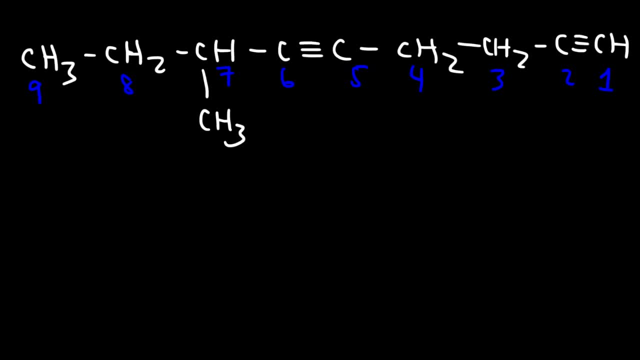 That's the longest chain, And so that's going to be nonane, But instead of nonane it's going to be non-9.. We do have two alkynes or two triple bonds, So it's going to be a di-ime. So let's put it all together. We have a methyl group on carbon-7.. So it's 7-methyl-3-hexime, And then we have a triple bond at carbon-1 and 5. So it's going to be 1,5-nana. 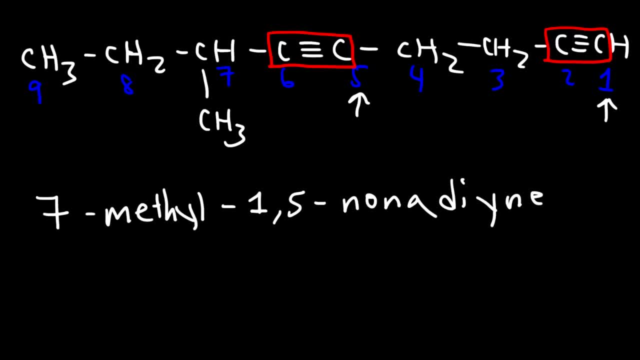 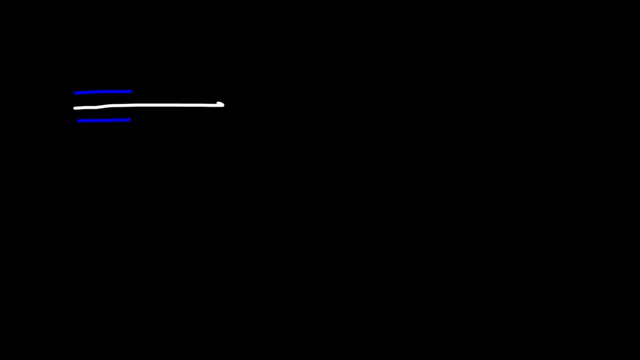 And then di-ime, because we have two triple bond functional groups, And so this is how we could name this particular molecule. Now, What do you do When you have a molecule that contains an alkyne functional group and an alkene functional? 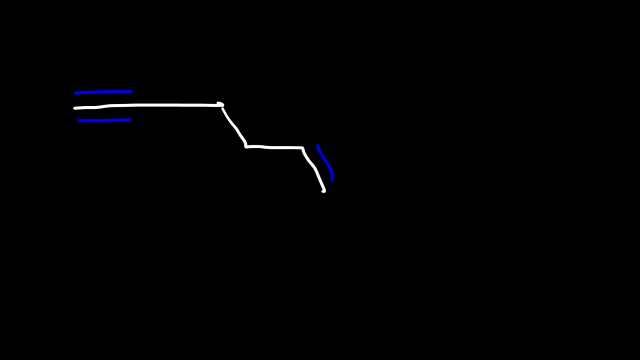 group. Which one has more priority? Should we place the one at the alkyne or at the alkene? In a situation such as this, the alkene has more priority, So we're going to count, given the alkene the lower number. 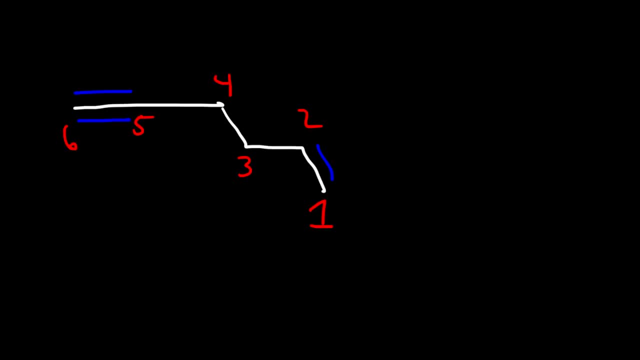 So we have 6 carbons. So this is hexane, but it's going to be hexene instead. Now, the way you name it, it's going to be 1-hexene, because the alkene is at carbon-1.. 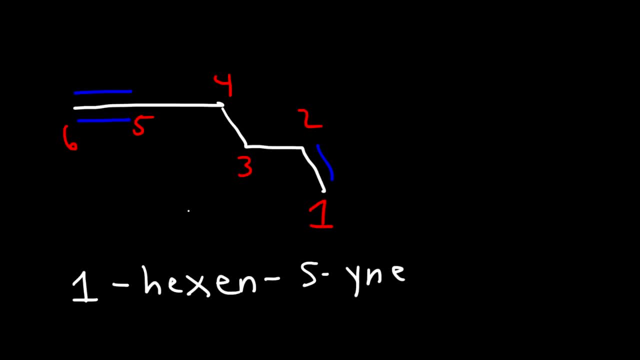 And then dash 5-ime, because the triple bond is on carbon-5.. And so that's how we can name a molecule that has an alkene and an alkyne functional group. Now what if we have an alkyne with an alcohol functional group? 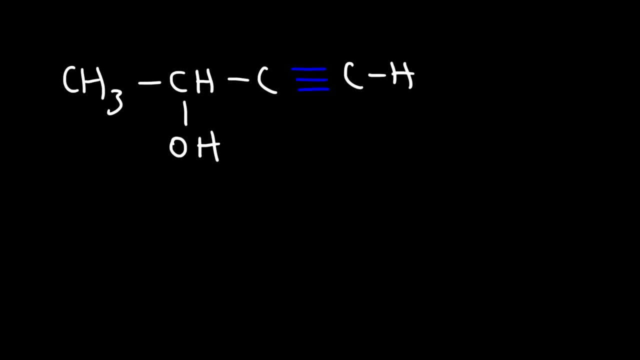 Which one has more priority, the alcohol or the alkyne. It turns out that the alcohol has a higher priority than the alkyne, So we're going to give the OH group the lower number. So this is called 3-alkyne.